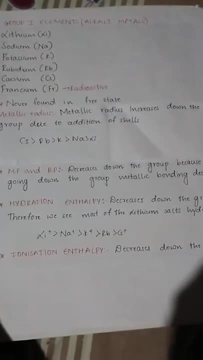 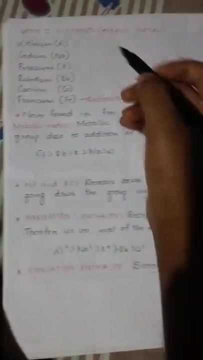 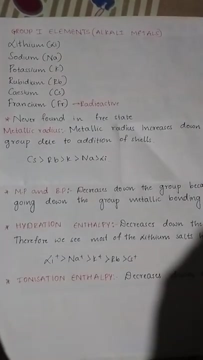 Today we will learn about group 1 elements, also called alkali metals. Here are group 1 elements: Lithium, Sodium, Potassium, Rubidium, Cesium, Francium. These group 1 elements are never found in free state because they tend to lose their Ns1 electrons very easily. They 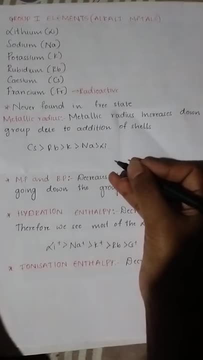 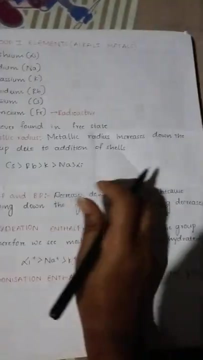 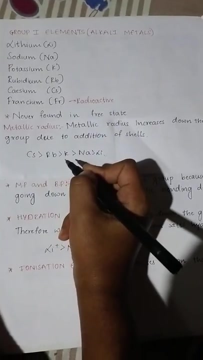 react with the other elements and form salts. That's why they are found in their salt state instead in their free state. Metallic radius. Metallic radius increases down the group due to addition of salts. Cesium has the more metallic radius than any other element in. 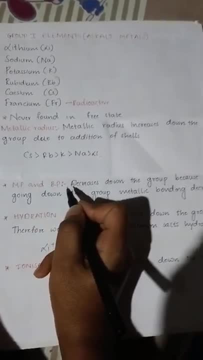 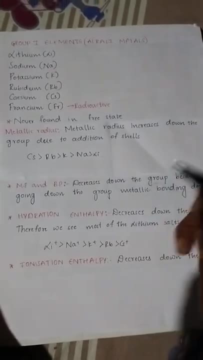 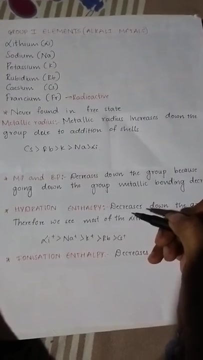 the alkali metals Melting point and boiling point. Melting point and boiling point mostly depends on the metallic bonding and the metallic bonding decreases down the group. That's why cesium has the least melting and boiling point. Lethium has more boiling and melting point. 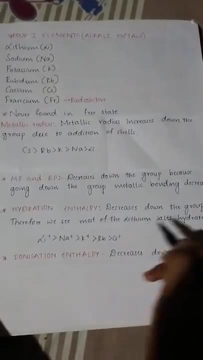 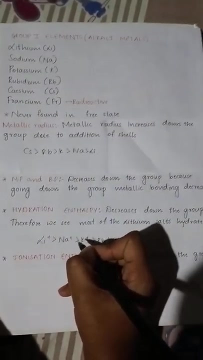 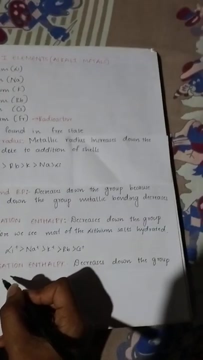 Hydration enthalpy, It decreases down the group. therefore, we see most of the lithium salts hydrated And Lithium has more hydration enthalpy than any other elements in group 1. elements: Ionization energy. When we come to ionization energy, it decreases. 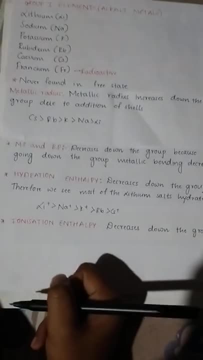 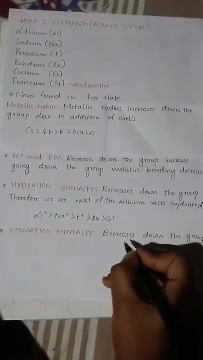 down the group. Ionization energy is the minimum energy needed to get the outermost electron or the most loosely bonded electron from the gaseous isolated element, ion or molecule. 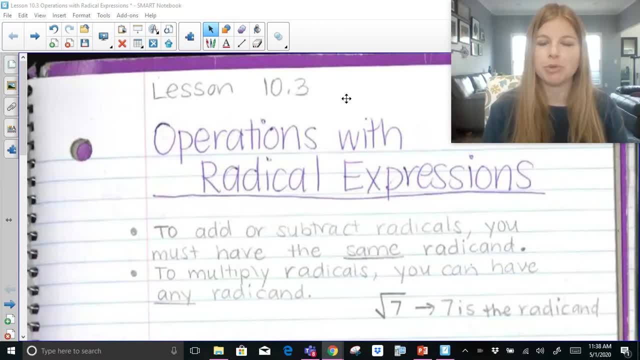 Hi everyone. today we're going to be talking about operations with radical expressions. We're going to be looking at adding and subtracting with them, but also multiplying. So follow along with me. If you don't know how to simplify radicals yet how to break down, let's say radical 20,. 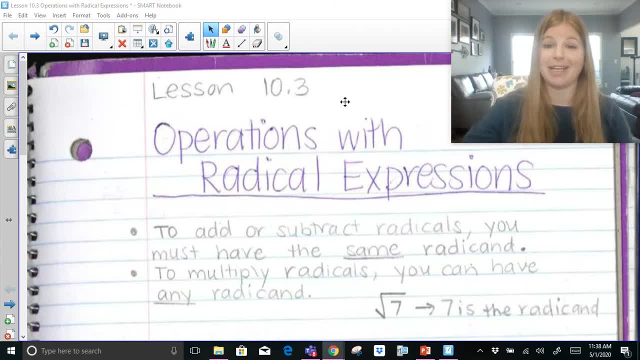 make sure you watch my other video so that you know how to do this before we get started. All right, so here's the rule that's on the screen. It says: to add or subtract radicals, you must have the same radicand.